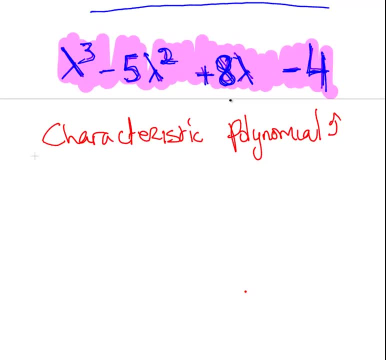 not easy, but like a sort of clue became evident. Now, what I'm going to do is work on the basis that there was no sort of obvious clue. Okay now, first off, just going to remark, this is a polynomial of degree 3. So we expect three roots to this, Okay. so three roots Okay, so that's to say three possible values for lambda that solve that equation, that are consistent with that equation. 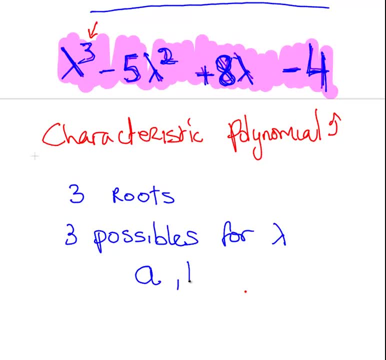 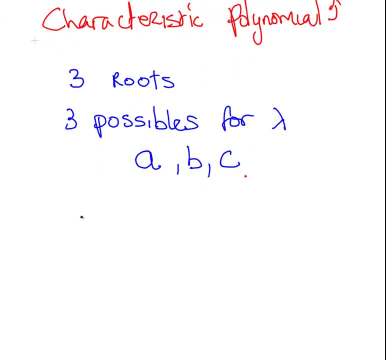 Okay, and what I'm going to call them is a, b and c, just for the time being. Okay, so if a, b and c are the roots for an equation, that means lambda equals a, lambda equals b, lambda equals c. Okay, now we might rewrite what I've just written there, this as follows: Okay, lambda minus 1 equals 0, or lambda minus a equals 0.. 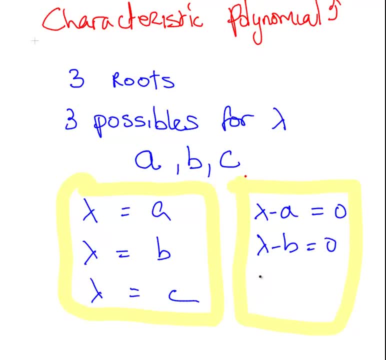 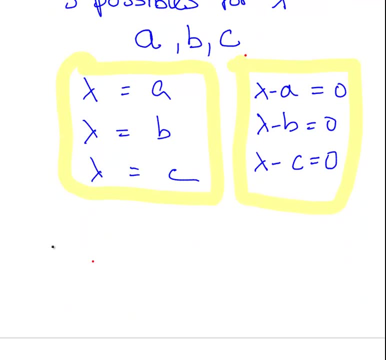 Lambda minus b is equal to 0, and lambda minus c is equal to 0.. Okay, now, if we have, essentially, if we're writing this as a polynomial- which, that is, those a, b, c are the roots for what we would do is write it like this: 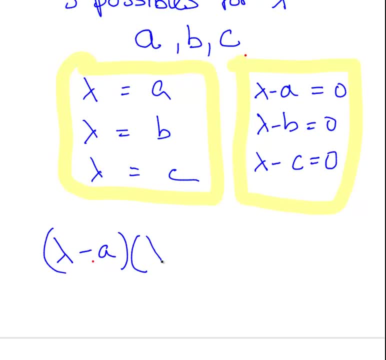 A minus, or lambda minus a, is equal to 0, lambda minus b is equal to 0, lambda minus c is equal to 0.. Oh sorry, lambda minus a times lambda minus b, times lambda minus c, that is equal to 0.. Okay, now that's a sort of important juncture. 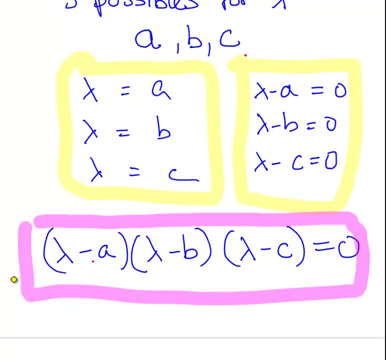 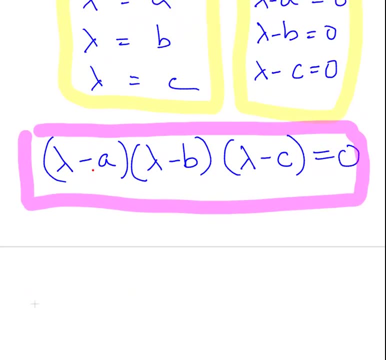 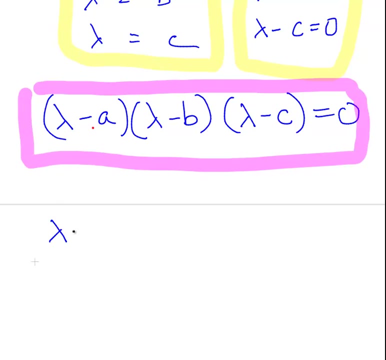 This part here. Essentially, this is the form that a characteristic polynomial will take For a 3x3 case if in a 4x4 case there will be 4 of them. Okay, now, what I'm going to just sort of remark upon here is I'm going to bit by bit calculate this out. So leave lambda minus a alone for the minute. 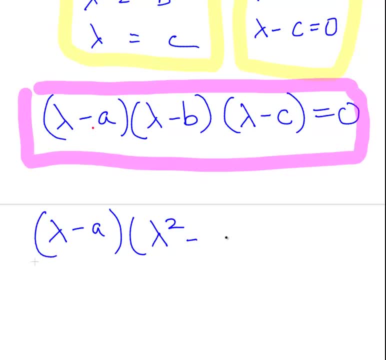 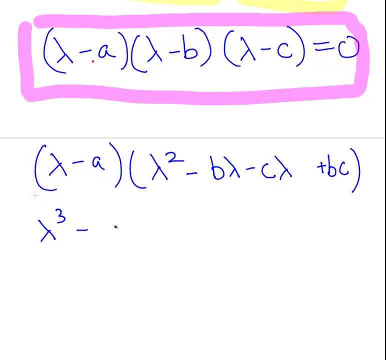 And what we have here is lambda squared minus b. lambda minus c, c. lambda plus b, c. okay, and when I calculate that out a little bit more, what I would get is as follows: lambda cubed minus b minus c. I'm going to put the plus there and put that in. 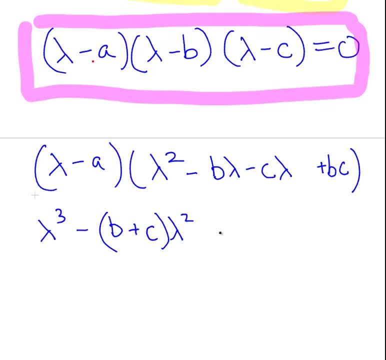 brackets: lambda squared- uh. minus, uh, or plus b c times lambda, and likewise minus eight times lambda squared- uh. well, it's actually plus, but I know that plus minus, but I'm going to actually just reverse the order there. sorry, just a little bit of digression there. 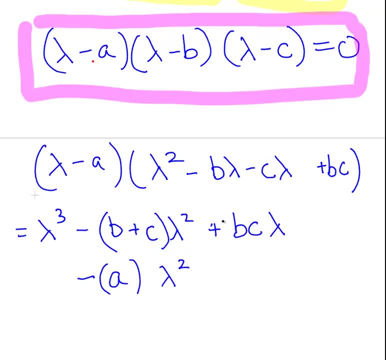 sorry, just a little bit of digression there, just make it easier to add it later on: uh minus a b, uh minus a times uh, plus. there we go. uh minus a times c, lambda and so on. but the last bit is most important. it's actually I'm just multiplying it out, but the last bit is a, b, c, essentially what? 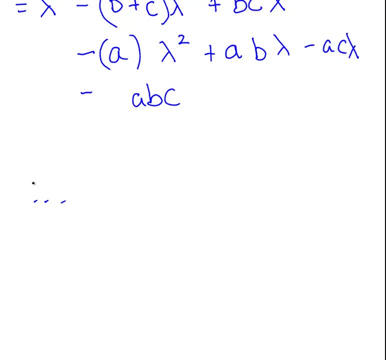 I'm going to say that getting getting out here is as follows: that this would be equal to lambda cubed, and then you have all the other terms in the middle which I'm not really particularly interested in, minus a, b, c. okay, so the first term is lambda squared- okay, that's fine, or lambda cubed, but the last term is what I'm specifically. 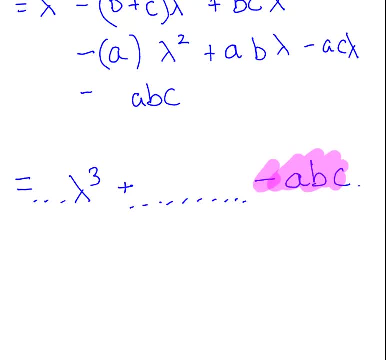 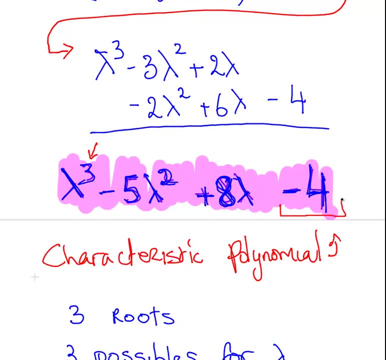 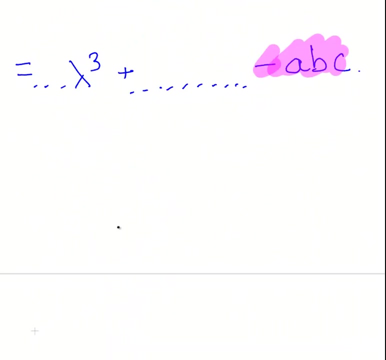 interested in a b c. minus a b c. okay, so minus a b c. so essentially, what I'm going to do now is try solve this here, this, uh get the roots for this. but what I'm going to sort of remark upon first off is: uh, minus four, which I just had up there, is equal to minus a, b and c, or minus a times b times. 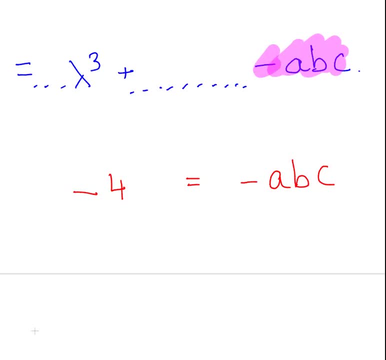 c, just as a remark. uh, so four is equal to a times b times c. now, just as a remark, what I'm going to do there is remark that, in the case of underprivileged numbers, I'm going to do is I'm going to do a graduate uh test where you've got about 15 minutes to get the eigenvalues they're usually going to. 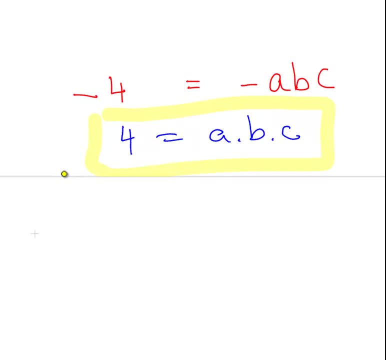 be integers not are close enough to integers you might get. I mean, you might get a square root or something like that, I don't know, but usually they're going to be integers, plus or minus integers. okay, so what we could do here is guess answers. okay, now the reason I'm going to sort of pick. 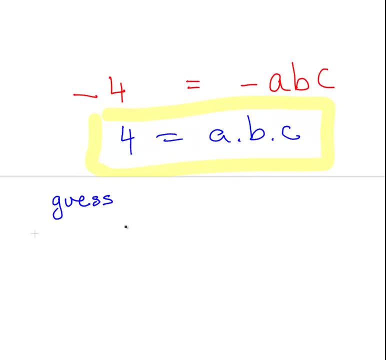 out a few and sort of suggest that they might be the answer, yes or no? well, first off, uh, in this case the answer is definitely not going to be, um, an eigenvalue. okay, because if we had a times b, times c, that means this other side would be zero. so zero is out, okay. how about plus or minus one? 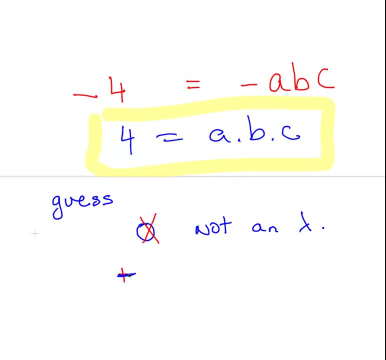 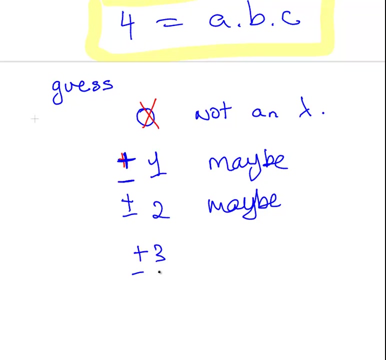 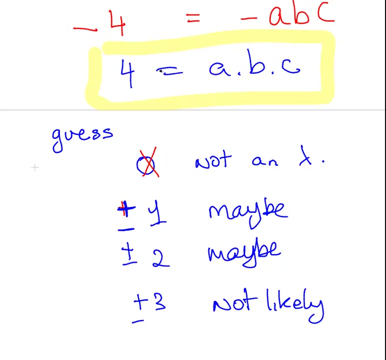 that's a potential case: plus one, minus one, maybe, likewise plus or minus two, maybe. uh, plus or minus two, maybe plus or minus three, maybe not, probably not, but maybe. so essentially, you're going to say that, no, not likely. okay. now the reason is: uh, three does not divide into four. okay, so what I'm going to do here? 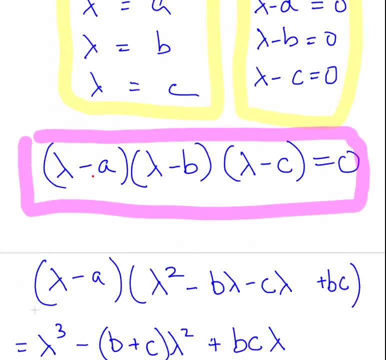 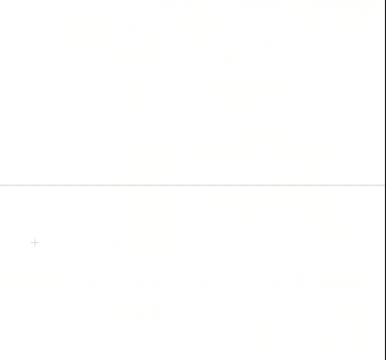 in this particular case is try out a few of these. uh, I'm going to try out this one here and what I'm going to do here- lambda cubed minus five. lambda squared plus eight. lambda minus four. we're going to try out a few trial solutions. 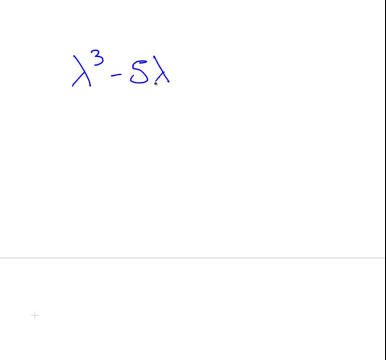 so source we're going to do is so: lambda cubed minus five. lambda minus four. we're going to do is order one over square root y lambda squared minus eight. lambda minus four is equal to zero. okay, let من் cin las school. lambda equal one, or we will get the answer. 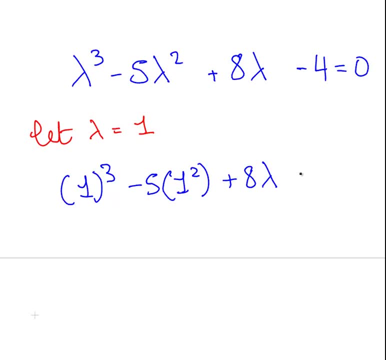 one cube minus times one square rootliay, eight times one minus four is equal to zero. so lambda cubed minus five, lambda squared plus eight, lambda minus five times one. we'll see what's going on here. end that 의 is equal to 0. that is, 1 minus 5 plus 8 minus 4 is equal to 0. yeah, that works. 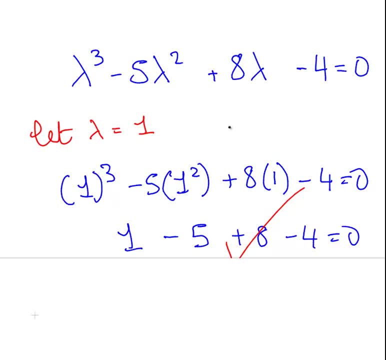 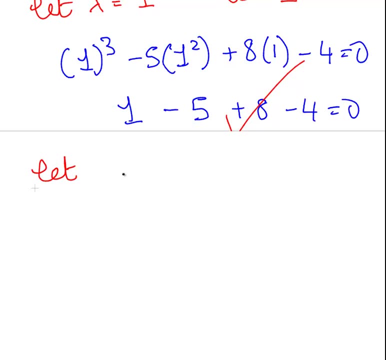 out. so we've actually found one of our values. we call that one a, so a is going to be 1, okay, so let's try out another one, and what I'll do here is you might be able to sort of do just a bit further. let's try out: let lambda equal to minus. 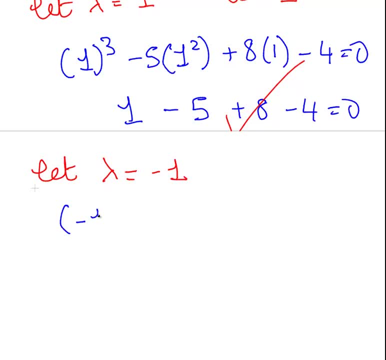 1 and see if this works okay. so minus 1, cubed minus 5 times minus 1, squared plus 8 times minus 1 minus 4, so this is minus 1, and so what we have there is minus 5 times plus 1, that's minus 5 minus 8 minus 4, not equal to 0. so this lambda. 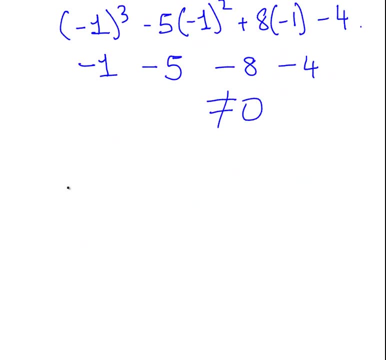 equals minus 1. no, okay, so we'll move on to lambda. equals plus 2, okay, so 2 squared, or 2 cubed minus 5 times 2 squared plus 8 times 2 minus 4. so what we have there, 8 cubed is. 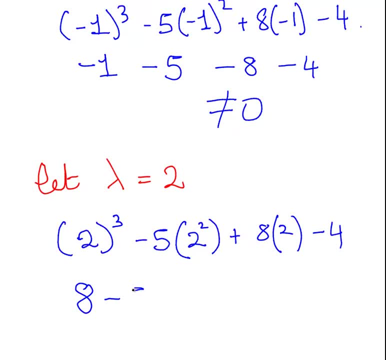 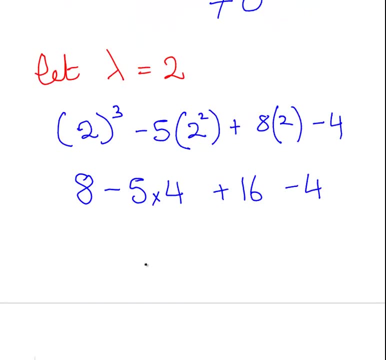 8, or sorry, 2 cubed is 8 minus 5 times 4, that's 20 plus 16 minus 4. that is equal to 8 minus 20 plus 16 minus 4, that's equal to 0. okay, so we've. 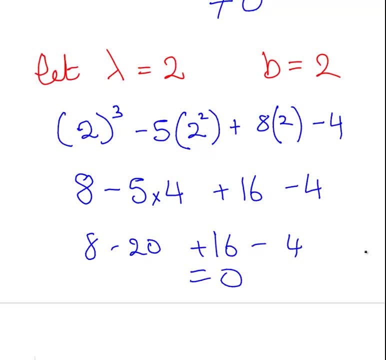 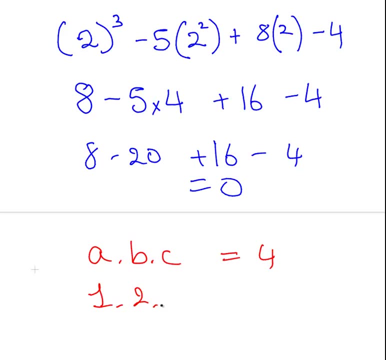 gone from the second one here, B is equal to 2. so, if remember, a times B times C is equal to 4. 1 times 2 times C is equal to 4. that means the last one is 2. so the eigenvalues that we are looking for, the solutions to the characteristic equation. 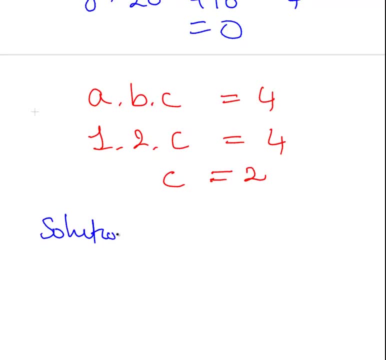 are the solutions to the characteristic equation and the solutions to the characteristics equation. the solution is a little bit more complicated, but i'm going to write this out fully. the solutions to characteristic equation or characteristic polynomial are as follows: one lambda equals 1, 2 and 2. okay, 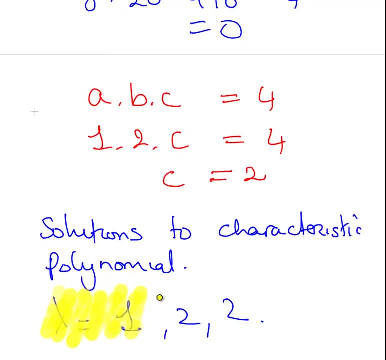 just a remark. I tend to write them in ascending order, not that it really matters, but it does sort of help to keep a consistent order when you're doing these sorts of things. so, correctly, that's a sort of a vector. but i'm just really the point, what i'm doing. 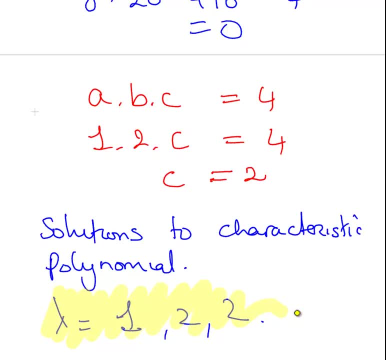 right now is solutions to the characteristic polynomial one, two and two.